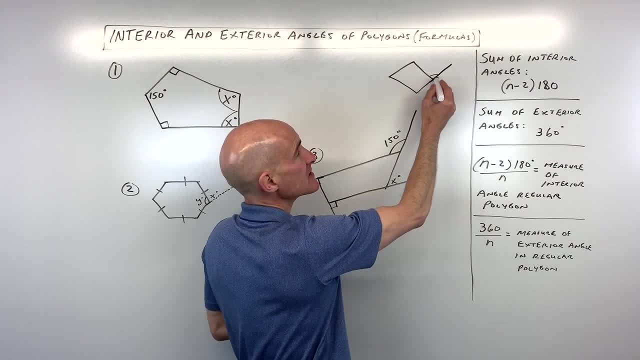 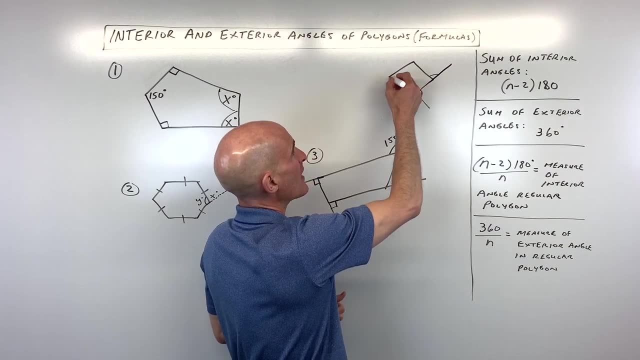 adding a number of angles to the polygon. you would add up to 360 degrees If you were just adding one of the sides that angle, there is an exterior angle. Same thing here if I was to extend either this side or this side, either one. that's an exterior angle. So you have one exterior angle. 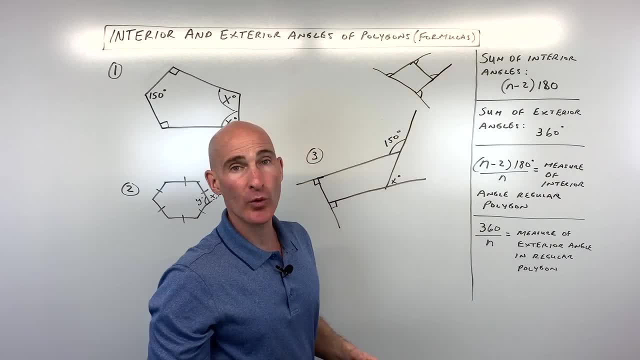 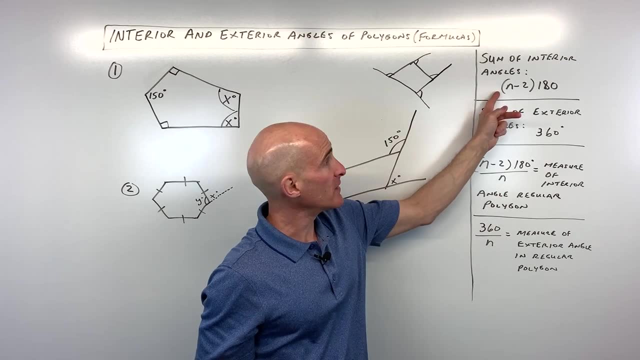 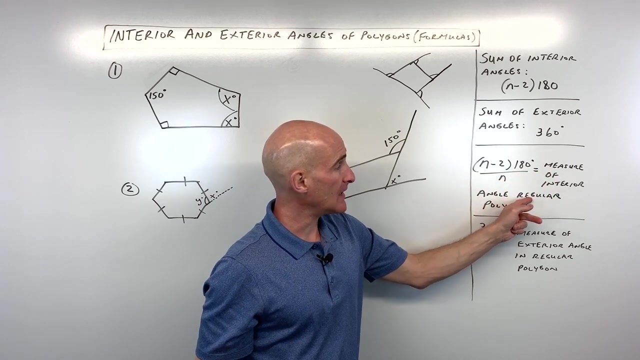 at each vertex, or at each corner, if you will, of the polygon. So all those angles would add up to 360.. This formula here is the same as this formula here, you can notice, but we're dividing by n and this is how you would find the measure of just one interior angle in a. 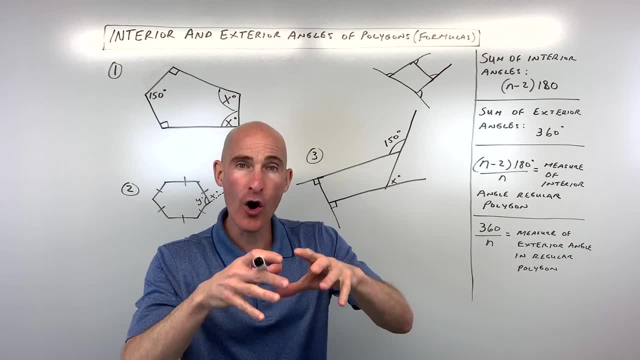 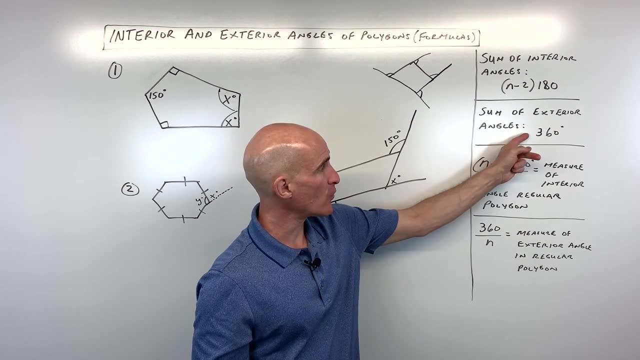 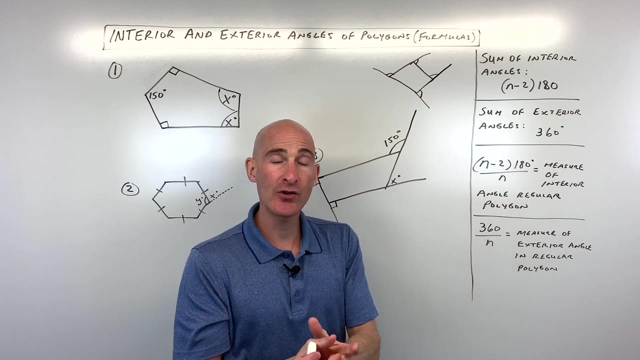 regular polygon. Now remember, with regular polygons all the angles are the same, all the sides are the same, And this last one here, 360, just like this formula, all the exterior angles add up to 360. But if it's a regular polygon, by dividing by the number of exterior angles, 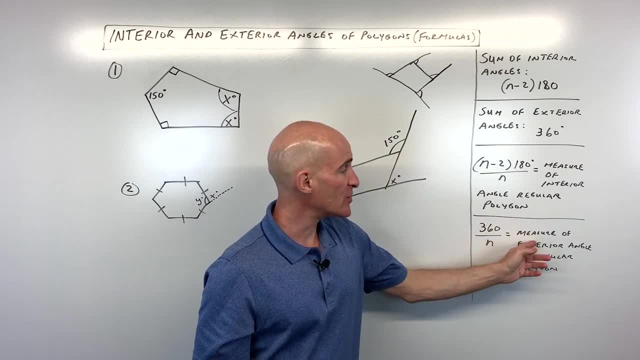 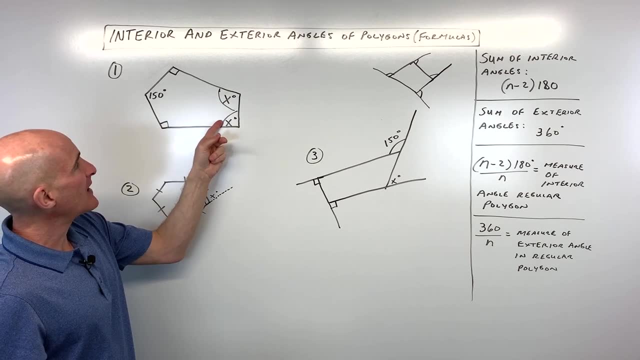 or by the number of sides. they're going to be the same. You can find out the measure of just one of those exterior angles. So let's go ahead and dive into some of these examples. Number one: how would you find out what these angles are? right here, Well. 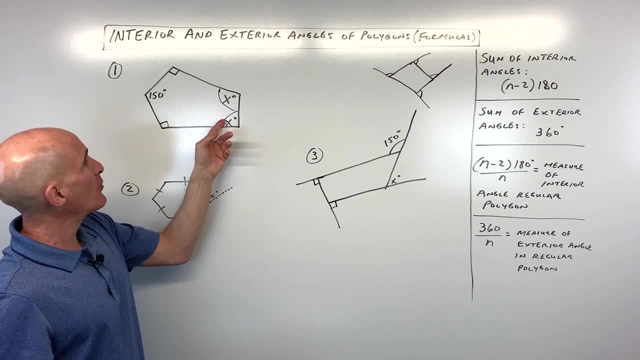 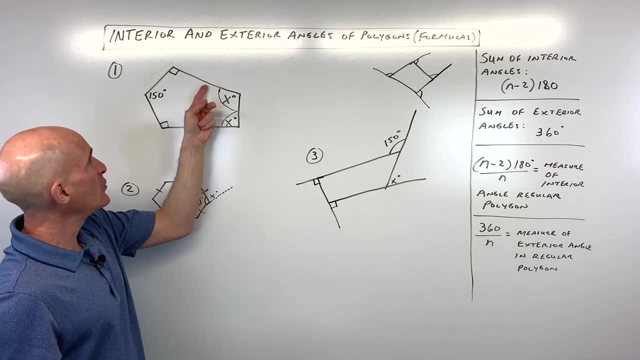 you can see they're the same, they're both x. But the first thing we have to figure out is: are these interior angles or are they exterior angles? Well, you can see, they're on the inside, they're interior, and we know that all these angles are going to add up to. 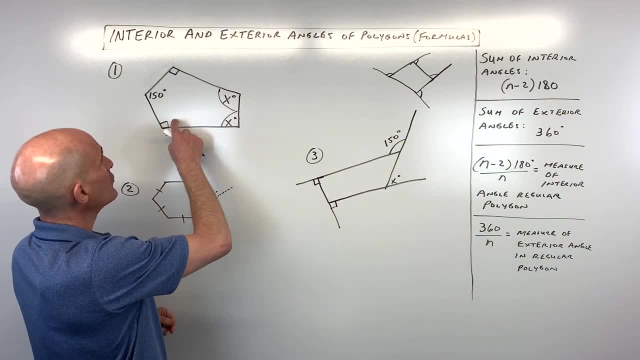 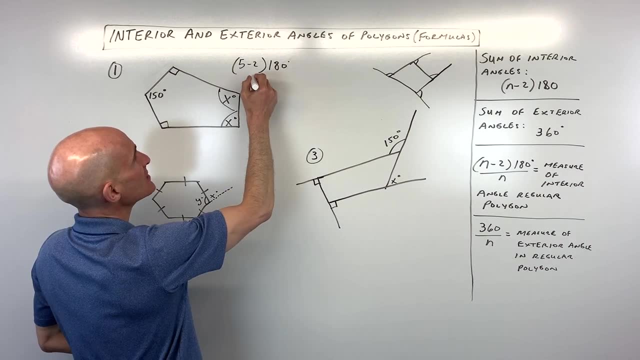 n minus 2 times 180.. Well, we've got 1,, 2,, 3,, 4, 5 angles, so it's going to be 5 minus 2 times 180 degrees. so that's going to be 3 times 180, which is 540 degrees total. 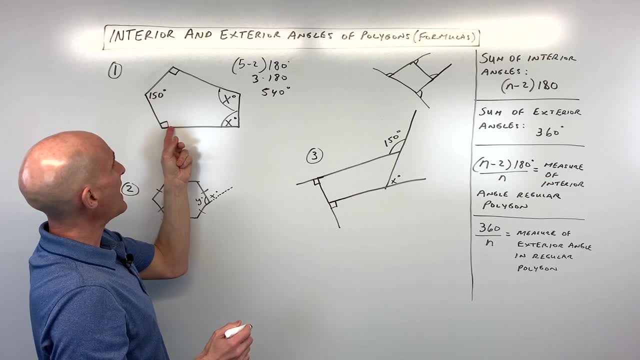 So if we add up all the angles- and this is what we're going to get- so if we add up all the angles, and this is what we're going to get- so if we add up all the angles, add these up: 90 plus 150 plus 90 plus x plus x, that has to equal 540, and we can write. 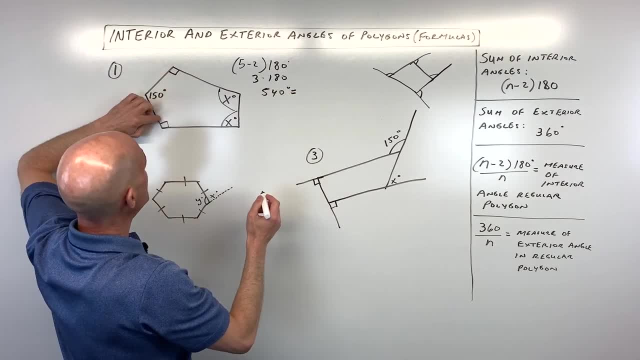 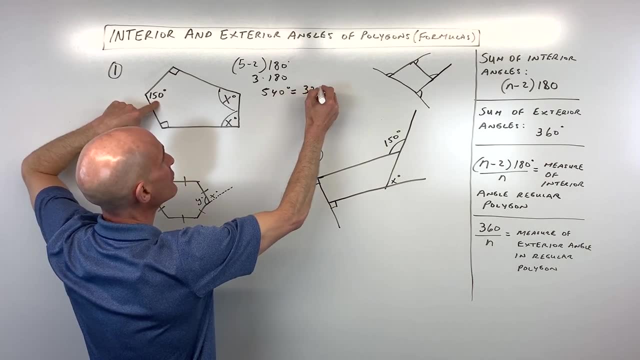 an equation. So let's go ahead and do that. Let's see: 90 plus 90 is 180, plus 100 is 280, plus 50 is 330, so that's 330, plus 2x equals the total of the interior angle is: 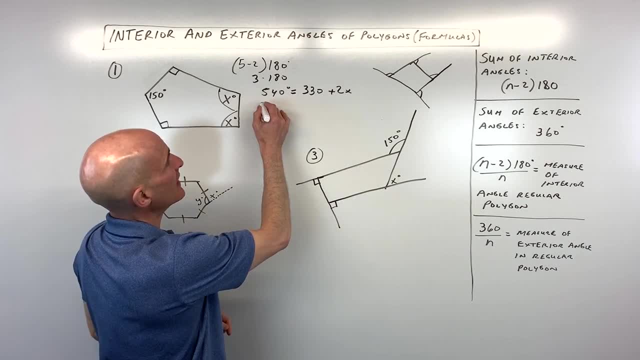 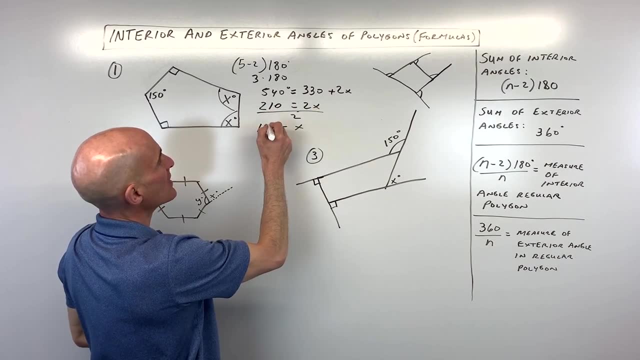 540.. If we subtract 330 from both sides, we get 210 equals 2x, and if we divide both sides by 2, we get x equals 105 degrees, and that's the measure of both of these angles. Okay, 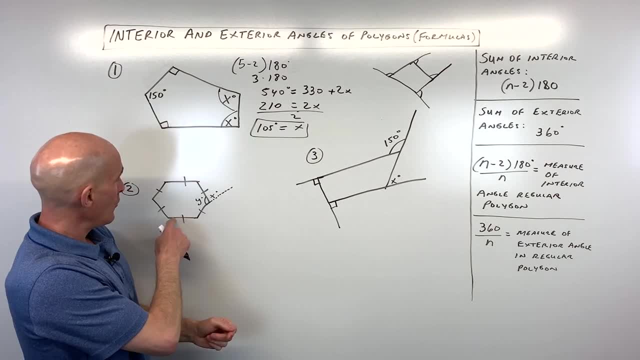 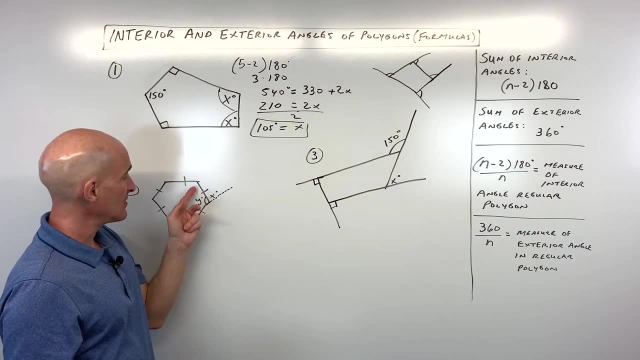 let's go to number 2 now. So for number 2, what we have is- we have see these marks here. all these sides are congruent. this is a regular hexagon, because there's six sides, six angles. all the angles are the same measure. all the sides are the same length. 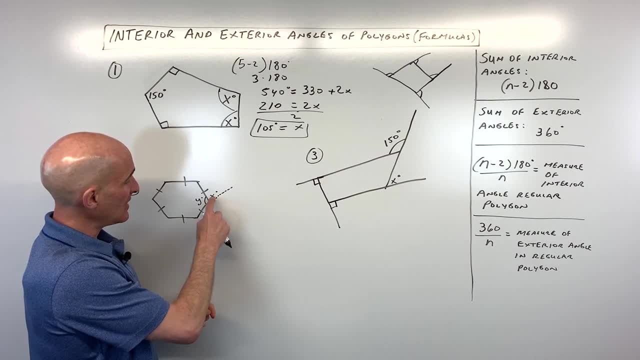 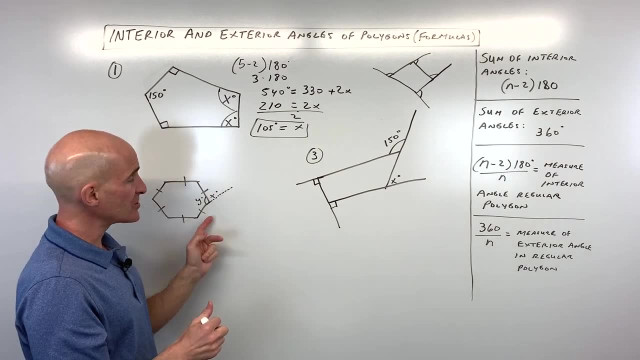 but what we want to do is we want to find out what the exterior angle measure is and what the interior angle measure is. So let's go ahead and find the. let's go ahead and find the exterior angle first. We know all the exterior angles add up to 360, but if 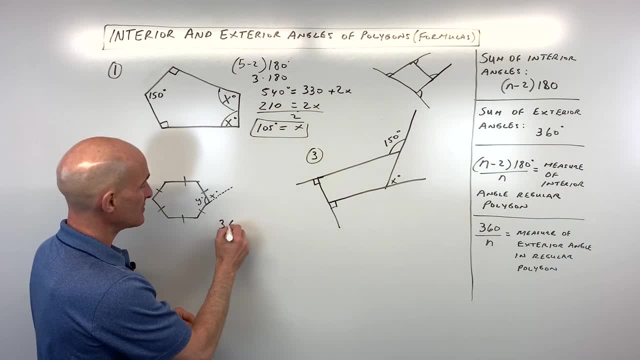 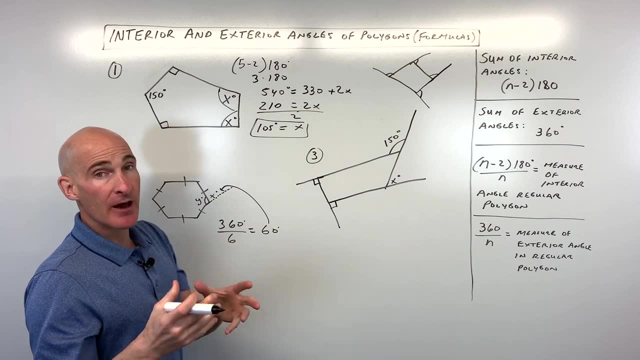 we divide by how many we have, which in this case is going to be 6, we get 60 degrees. so that's the measure of just this exterior angle here: 60.. Now to find the interior angle. you can see how this forms a straight line right here. So if this angle is 60, this angle. 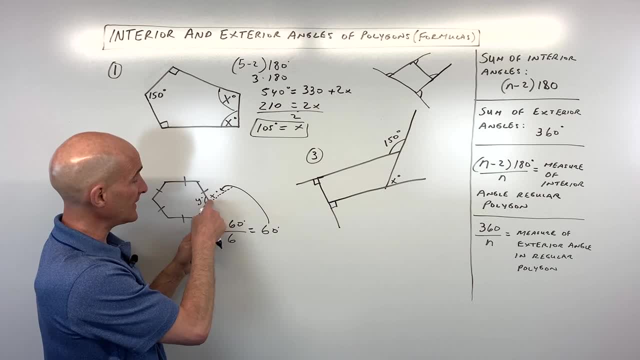 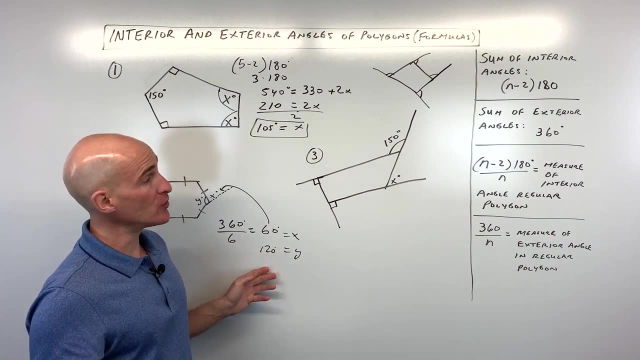 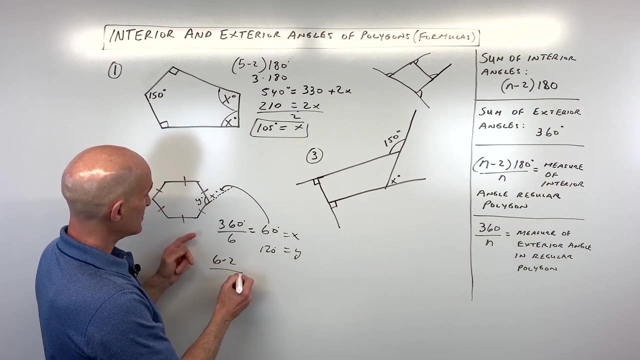 on the inside must be 180 minus 60, they form a linear pair, so that means that y is going to equal 160.. Now the other way to do it is to use this formula right here, and we can say n minus 2, so that would be 6 minus 2,, since there's six angles here, times 180,, so that gives 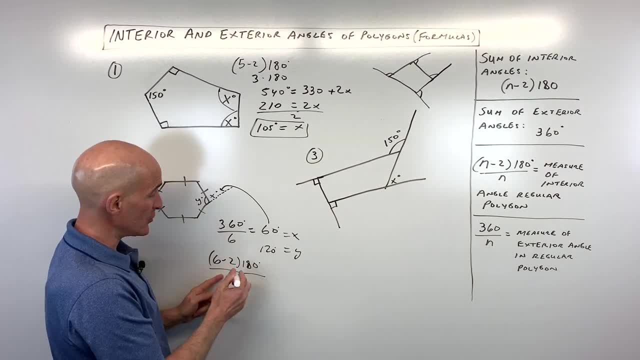 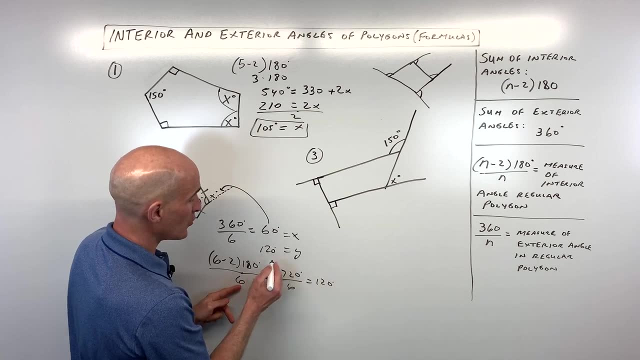 us 720, so that's the sum of all the interior angles. but then we're dividing by the six interior angles. so 720 divided by 6 equals 120, the same thing we got here. So sometimes it's easier to use this formula and then just subtract the interior angles and then 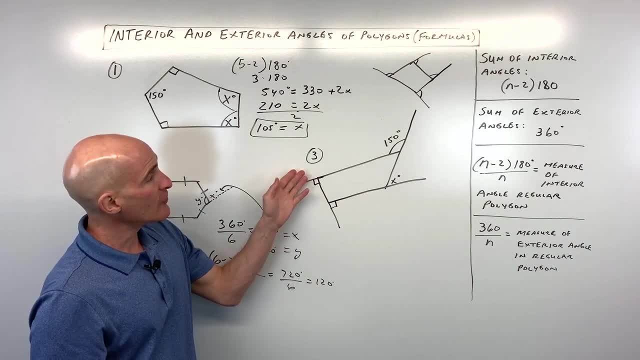 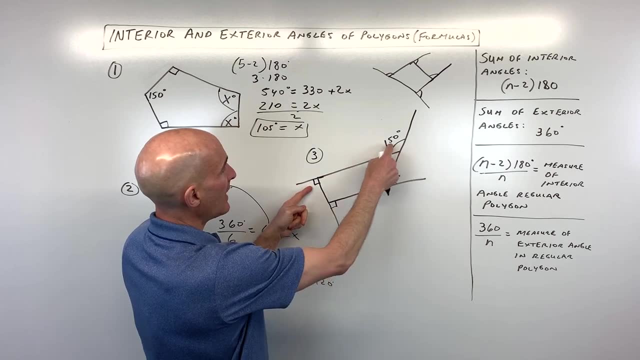 try, from 180 to find the interior angle just a little bit quicker. For number three. now, what do you think for this one? Well, it looks like we're given the exterior angles here, and we know that all those exterior angles add up to 360.. Now, this is not a regular. 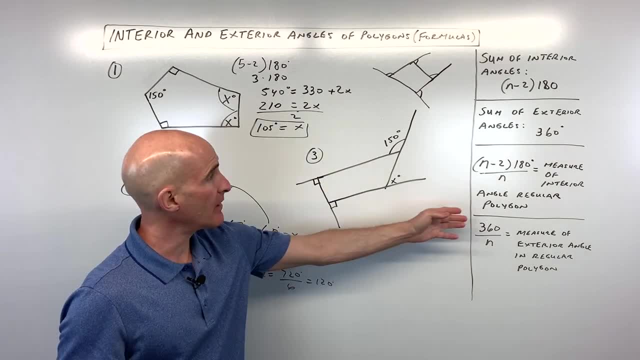 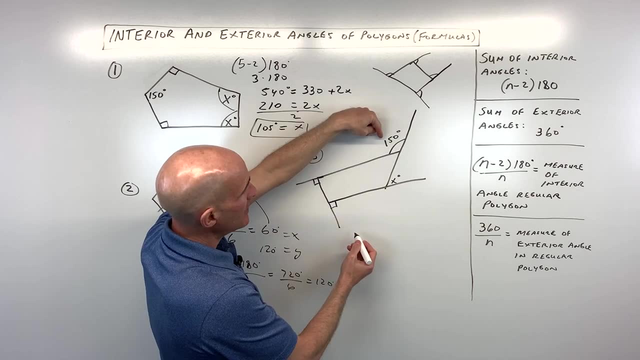 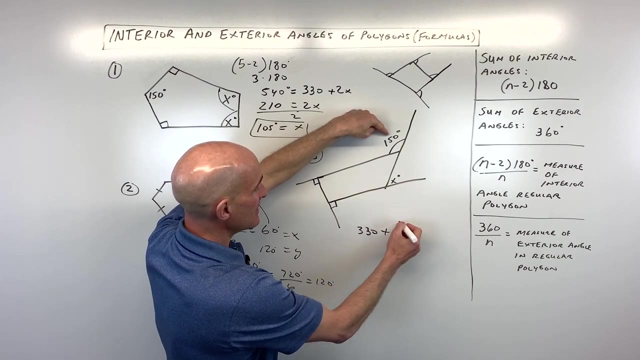 polygon, all the sides and all the angles are not the same, but they always add up to 360.. So let's just make an equation here: 90 plus 90 is 180, plus 150 is 330, and then plus x equals 360 degrees. So if we subtract 330 from both sides, you can see that x this. 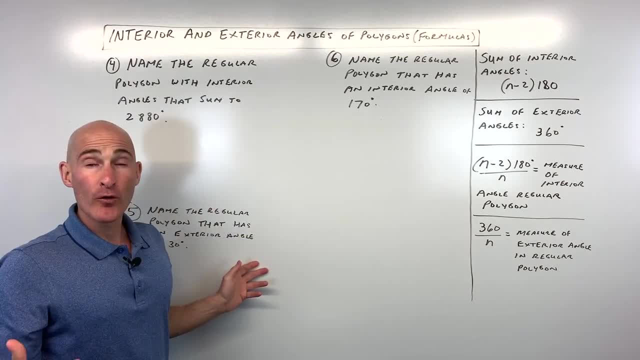 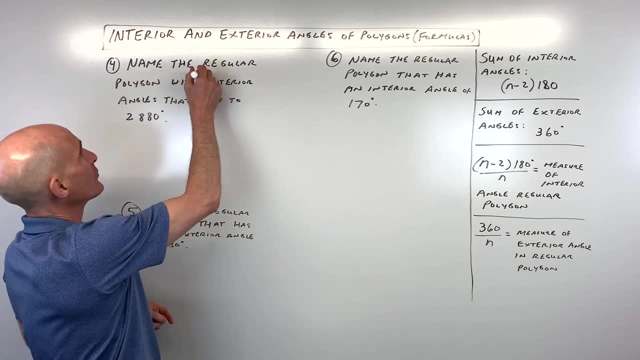 missing angle here would be a 30 degree angle. Okay, number four, five and six. these are like word problems. see if you can do these on your own and we'll go through them. Number four says: name the regular polygon with interior angles that sum to 2880 degrees. Okay, so, 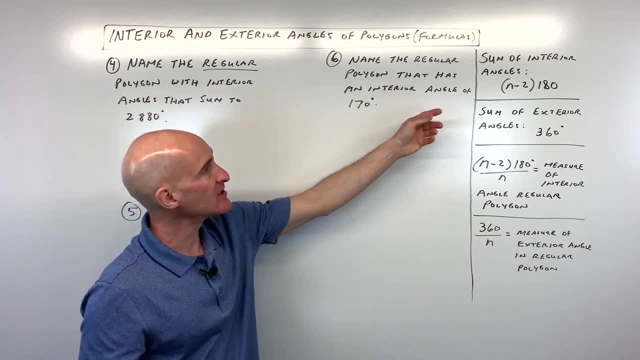 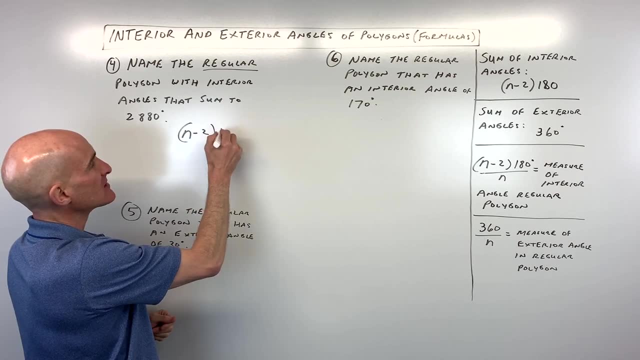 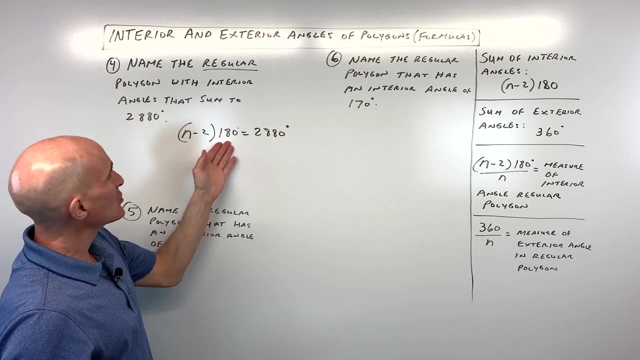 basically they're telling us, all those angles on the inside of the polygon add up to 2880, so we want to use this formula right here. it's gonna be: n minus two times 180, equals the total of the interior angles, which they tell us is 2880 degrees. So you can do this. 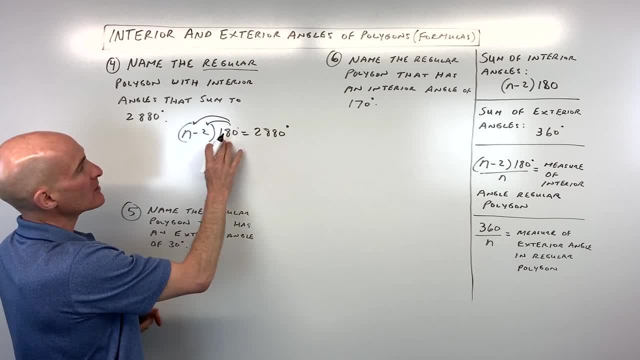 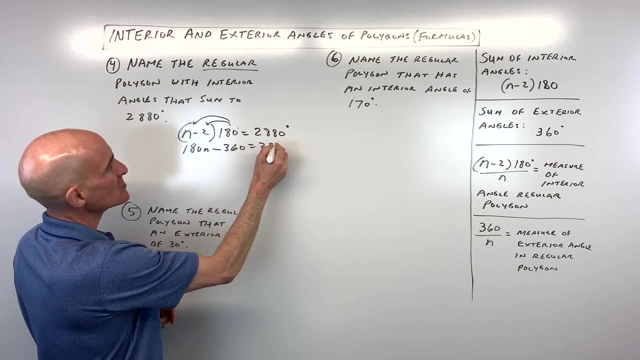 a couple different ways. you could distribute the 180 like this, or you could divide both sides by 180.. I'll just distribute. so this is 180n minus 360 equals 2880.. If we add 360 to both sides, 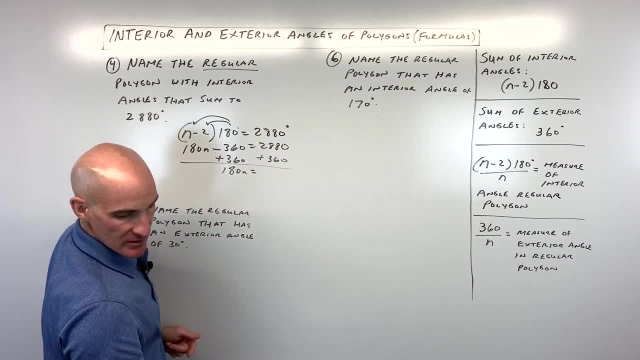 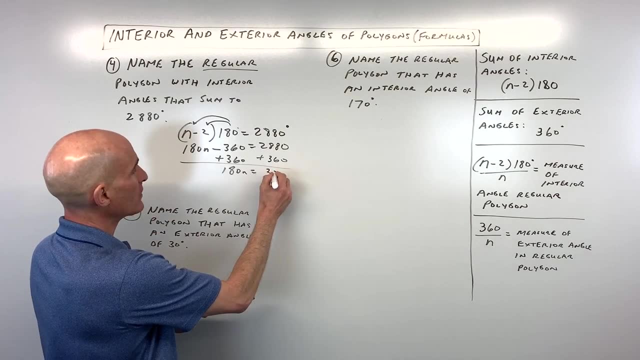 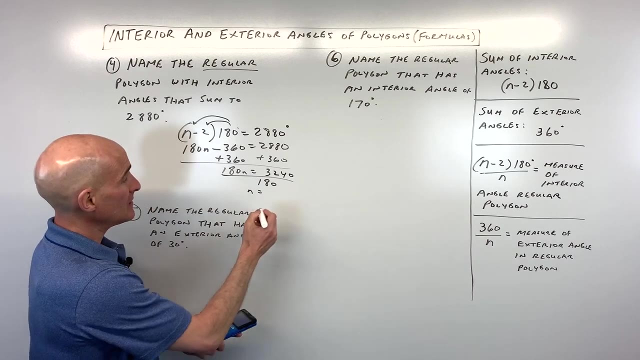 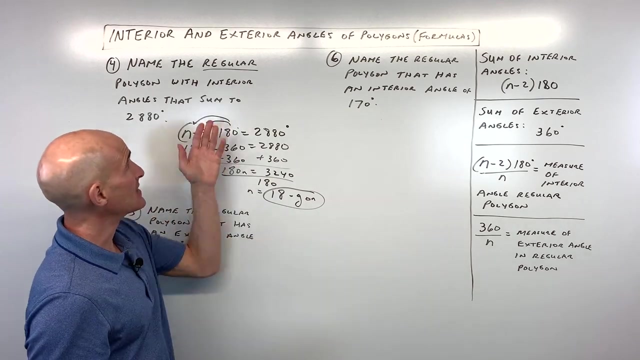 That gives us 180n equals- let's do this on the calculator- 2880 plus 360,, so that's 3240.. And if we divide both sides by 180, that comes out to 18.. So that means this is an 18-gon, meaning it has 18 angles or 18 sides, and it's a regular 18-gon. 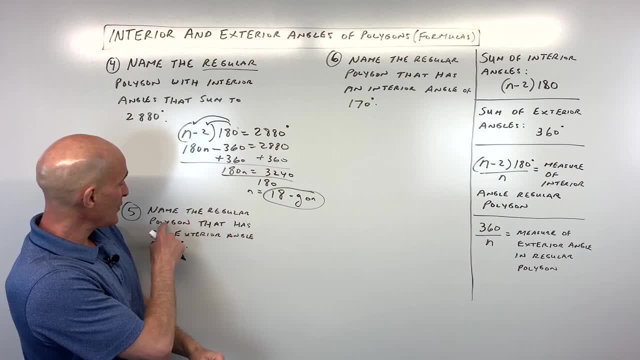 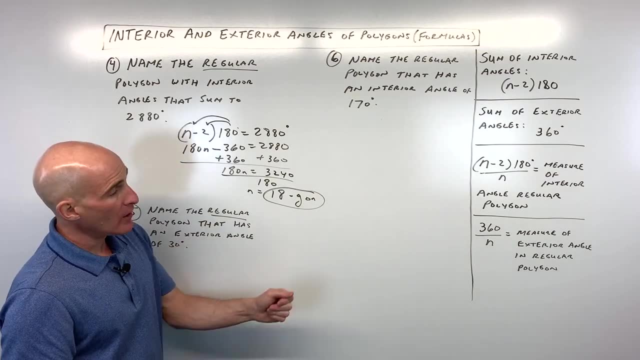 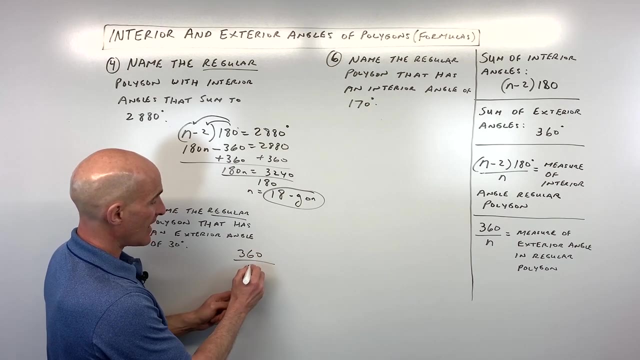 Okay, for number five. now it says: name the regular polygon, so another regular one that has an exterior angle of 30 degrees. Okay, so let's use this formula over here If we want to find the measure of just one exterior angle. it comes out to: 360 divided by n equals the measure of that exterior angle. 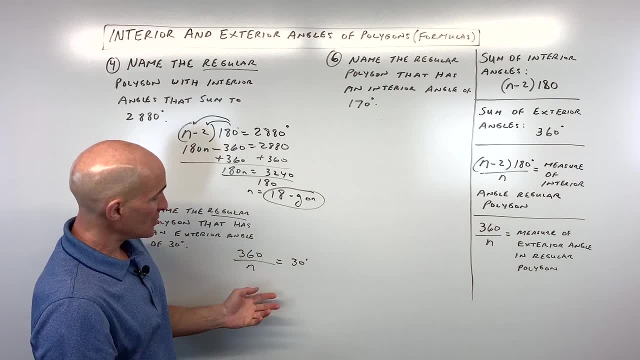 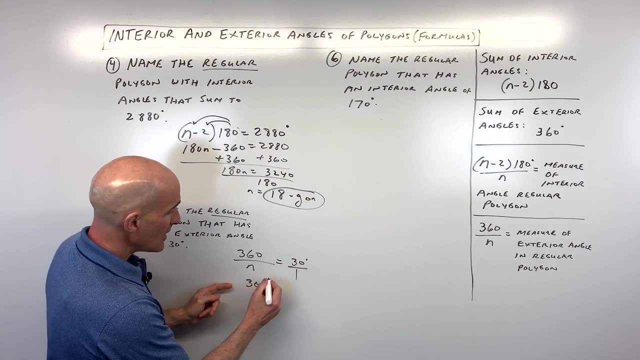 which in this case they tell us is 30 degrees. So what we can do here is we can think of this as 30 over 1, and we can cross-multiply on the diagonal. So this is the cross-product. So 30 times n equals 360 times 1, which is 360.. 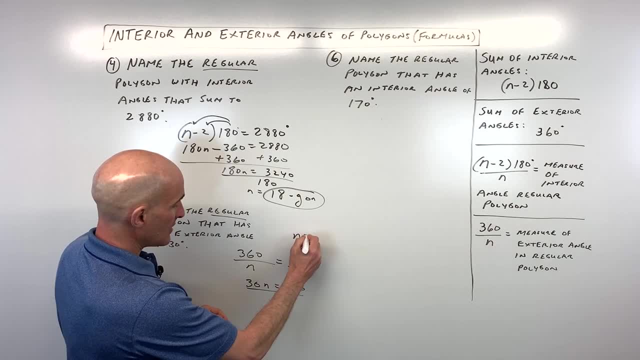 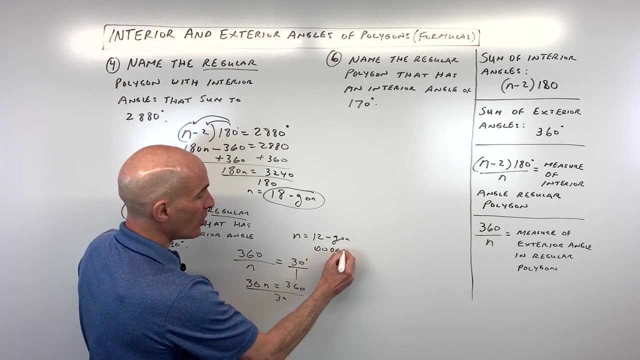 And if we divide both sides by 30, n comes out to 12.. So you could say this is a 12-gon, or this is also called a dodecagon. Okay, dodecagon. Decagon is 10 sides, dodecagon 12..